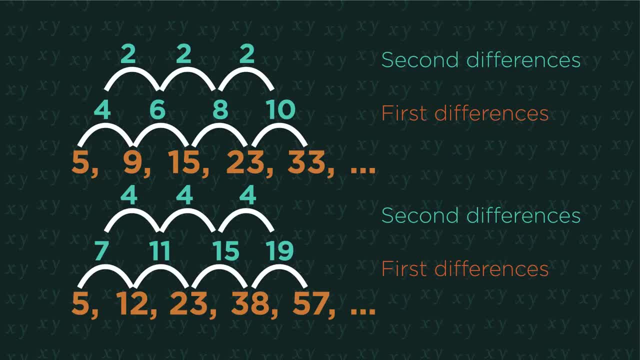 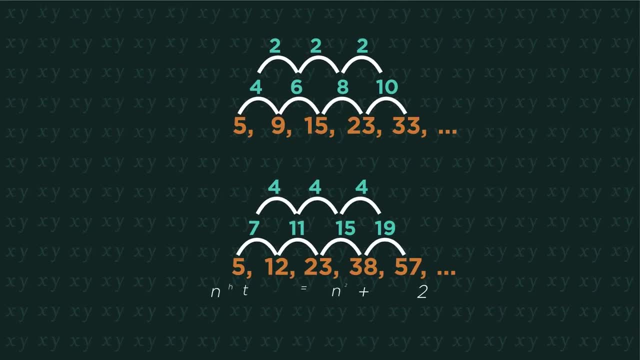 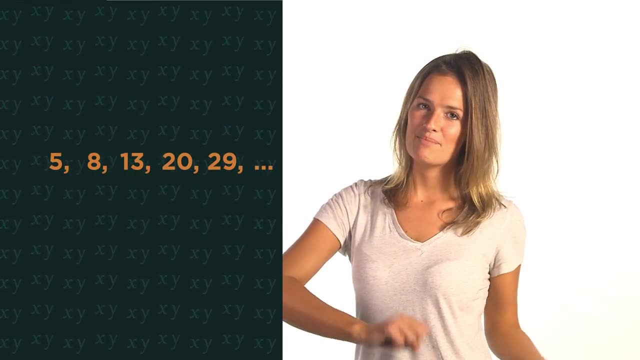 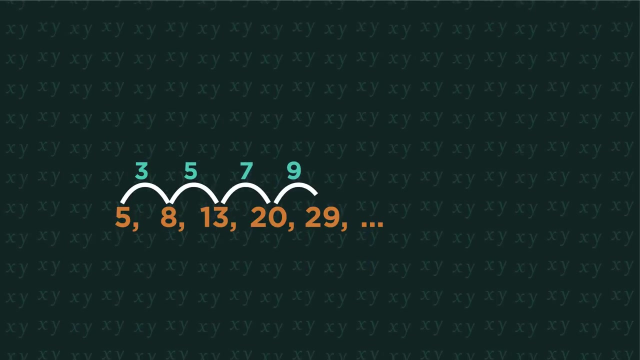 But now look at the second differences. If the second difference is constant, the sequence is quadratic. This means it contains an n squared term. So let's have a look at how to find the nth term of quadratic sequences. We have this sequence: Find the first and second differences. 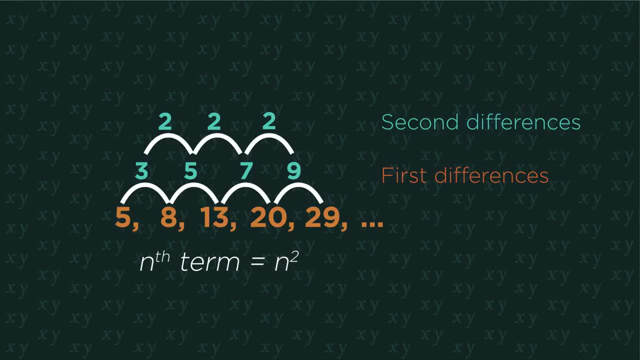 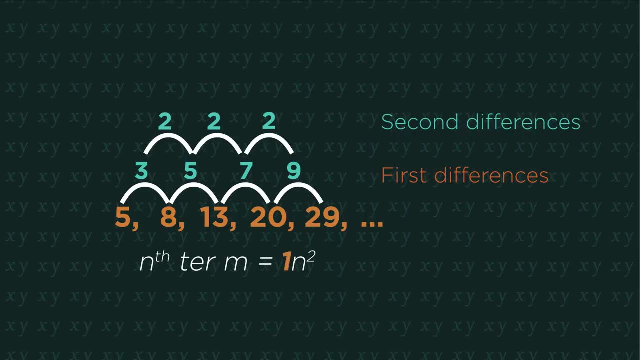 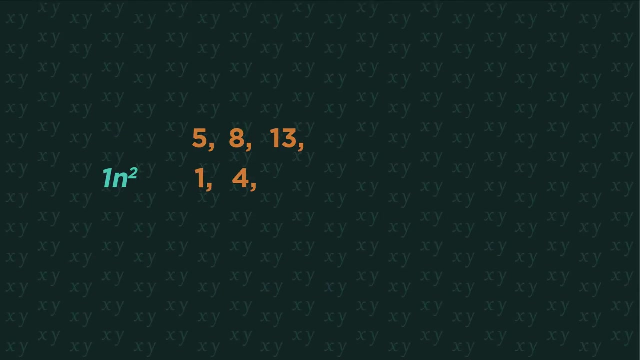 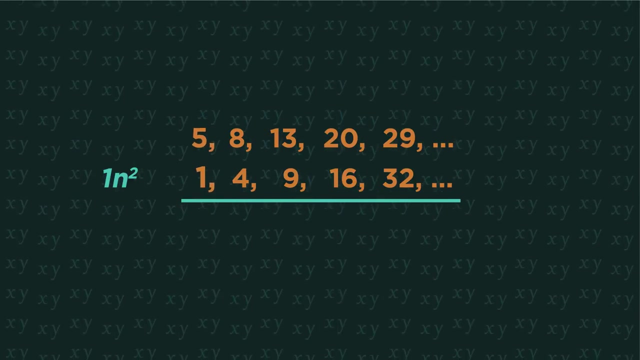 There's a constant second difference, so it's going to be n squared. Because the second difference is two, it will be one n squared, Always half the second difference. Now write out the original sequence and the one n squared underneath it. Compare the difference. So 5 to 1 is 4, 8 to 4 is 4, 13 to 9 is 4, and so on. 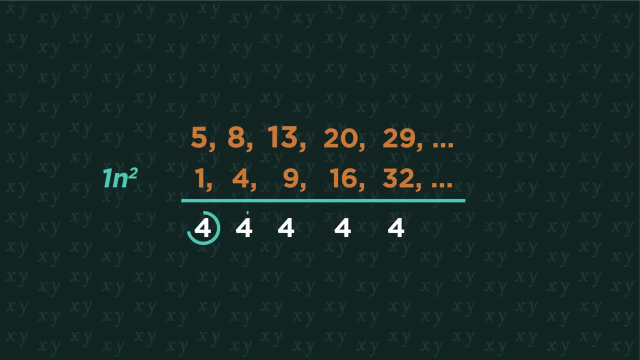 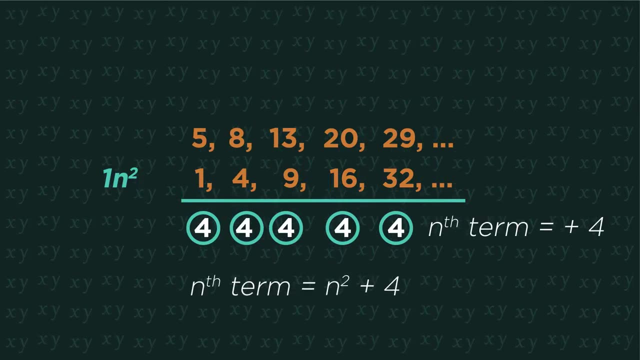 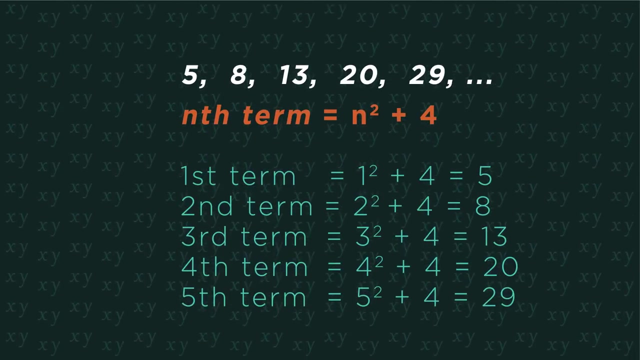 All you need to do is find the nth term of this sequence And you have your quadratic nth term formula. So it's n squared plus 4 for this sequence. As always, you should check it. So let's have a look at another one. 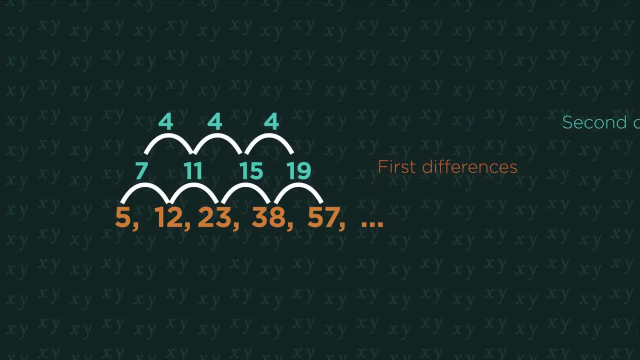 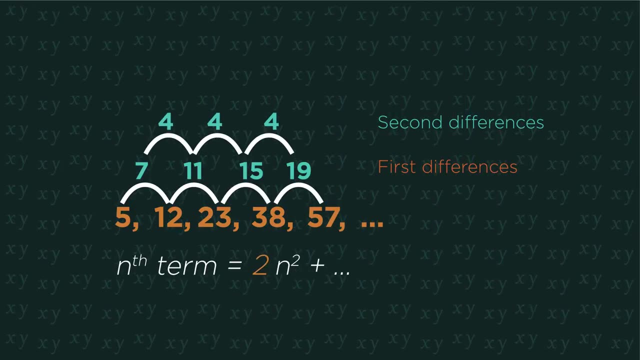 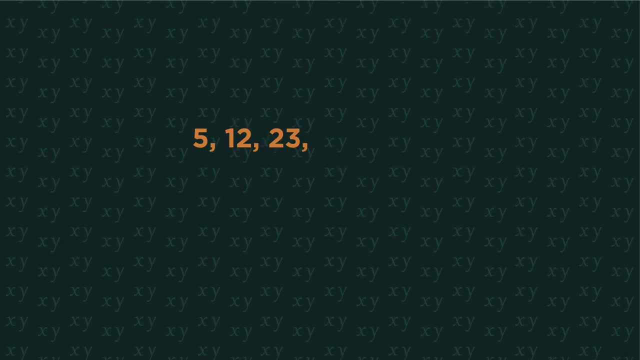 Find the first and second difference. Because the second difference is 4, the quadratic will be 2 n squared. Remember that we always half the second difference. Now write out the original sequence and, 2 n squared underneath it, Find the difference between the two. 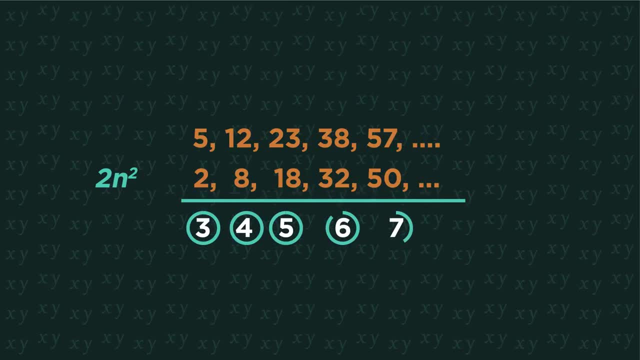 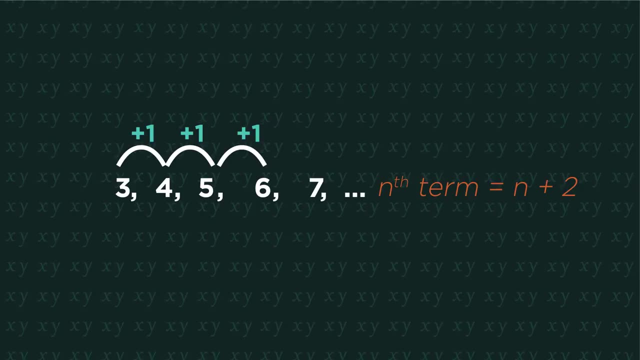 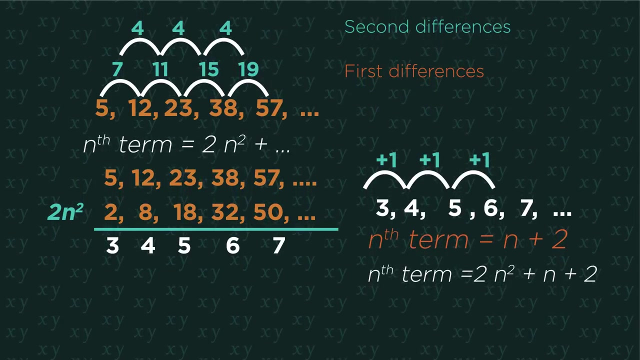 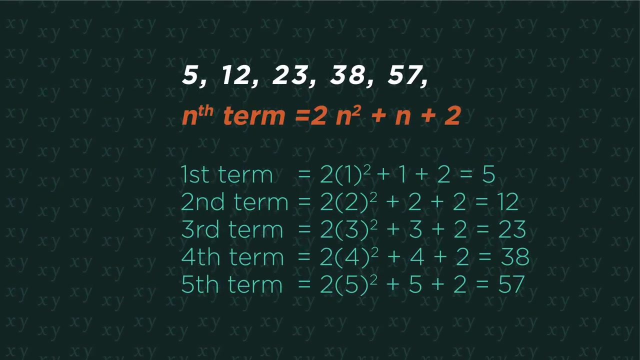 Now you need to find the nth term rule for this. It's n plus 2.. So the nth term rule for this quadratic sequence is 2 n squared plus n plus 2.. And, as always, check it. So here's two for you to do. Pause the video. find the nth term. 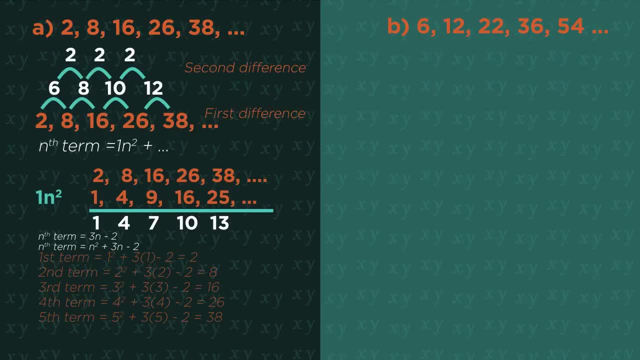 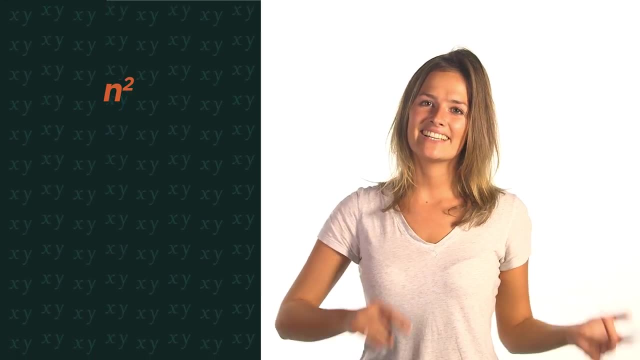 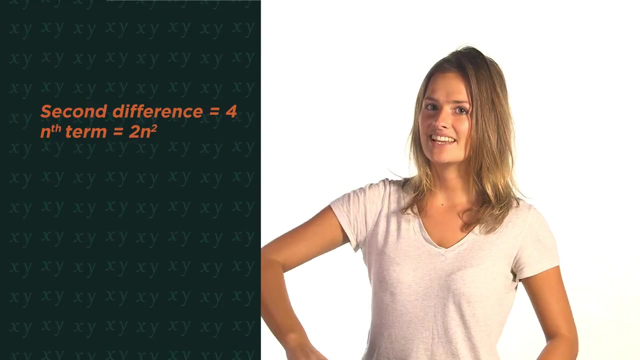 click play when you're ready. How did you do So? there we have, finding the nth term for quadratic sequences. Just remember to look for that second difference and then half it. If you have any questions, please comment below. like and share our videos with your friends.